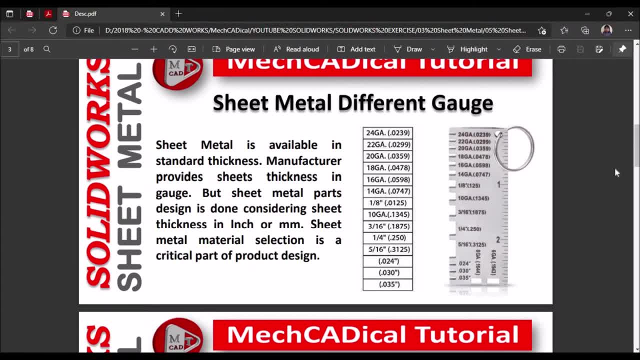 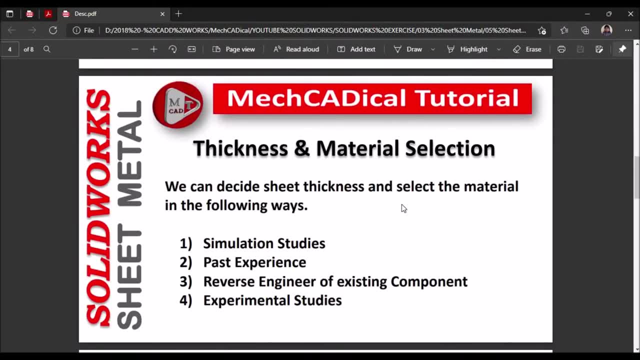 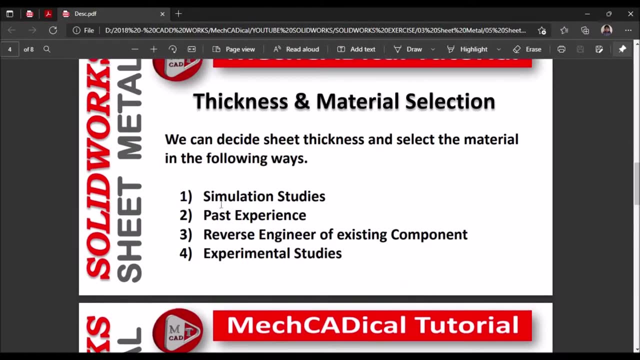 increase the gauge, the sheet thickness reduces. So based on our requirement, we can select our sheet metal thickness as well as the material. On what basis we define the thickness of the sheet metal thickness and material? So first method is simulation studies. Second, 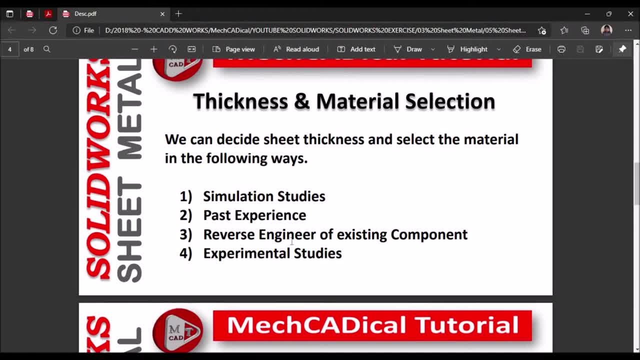 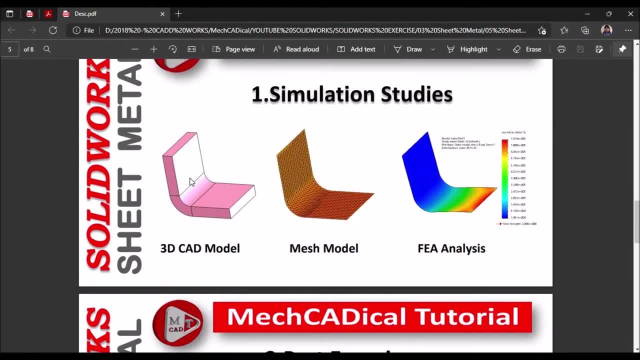 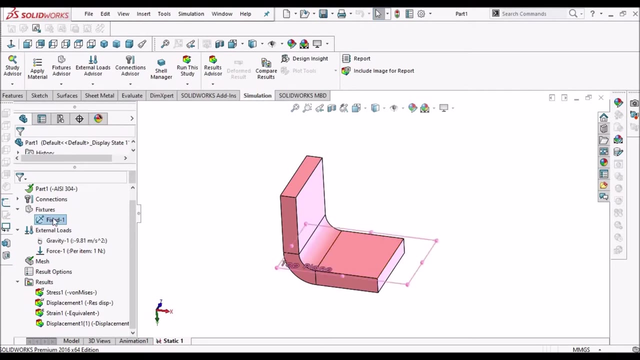 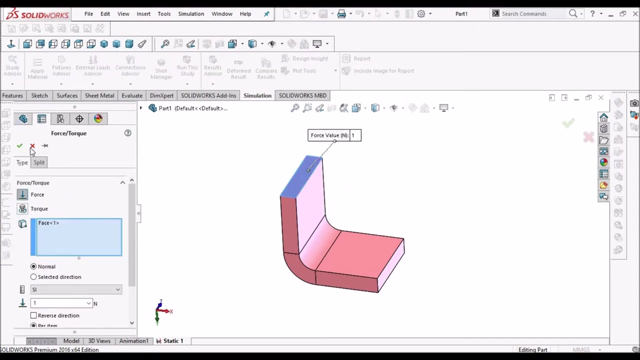 method is passed by past experience. Third method is reverse engineering of the existing component and experimental studies. So in simulation we create the CAD model, we apply the defined loads and we see the stresses and deformation, For example. this is the CAD model. I have applied the fixed load over here And this is the load applied on this. 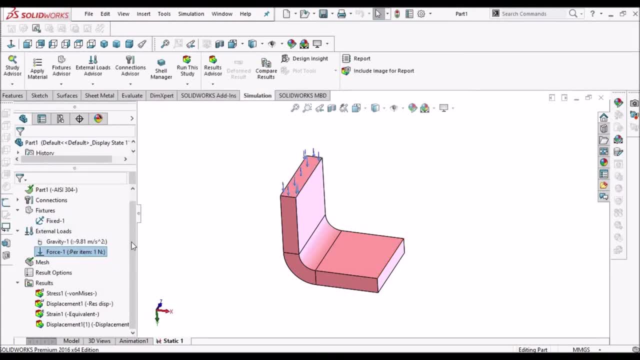 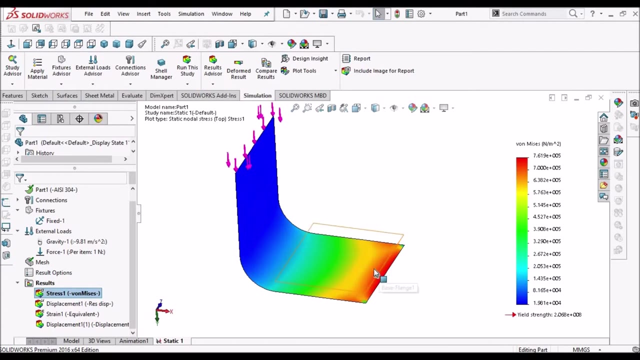 face. So what are the changes are happening? We will see the stresses and deformation In the component. So this is the stress developed and maximum stress developed over here: the red zone and medium stresses at this green zone and no stresses at this location. So 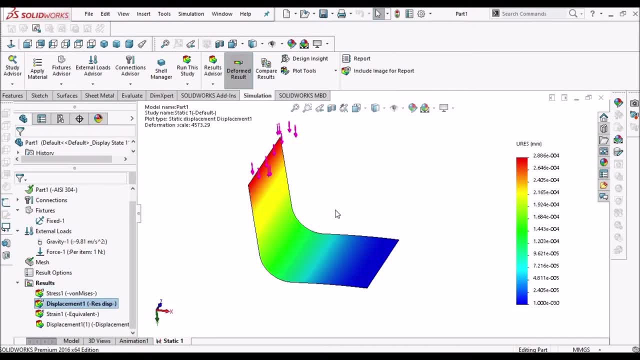 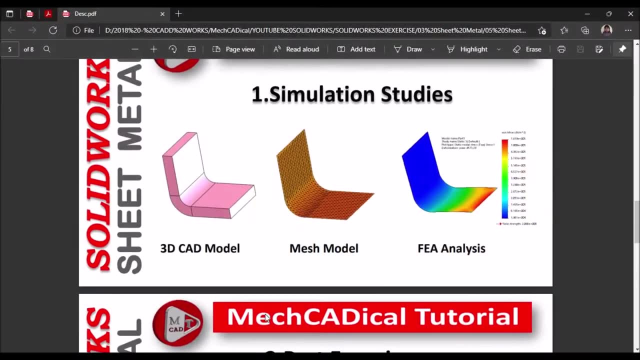 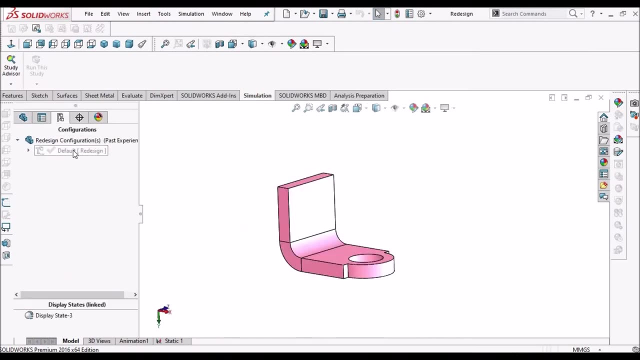 similarly we can see the deformation. Based on that we can modify the design of the component. So next method is by past experience. First, suppose we have a component. Suppose we have a component, This is the existing design And based on this existing design we can modify our design. 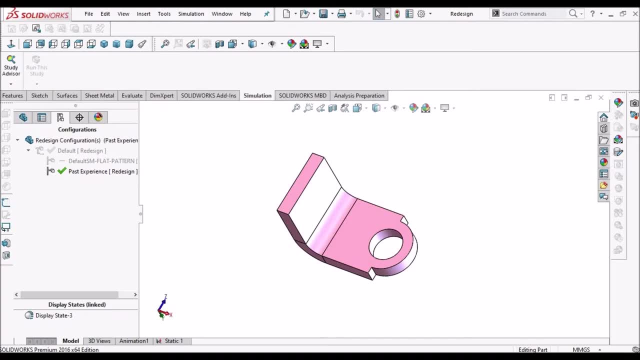 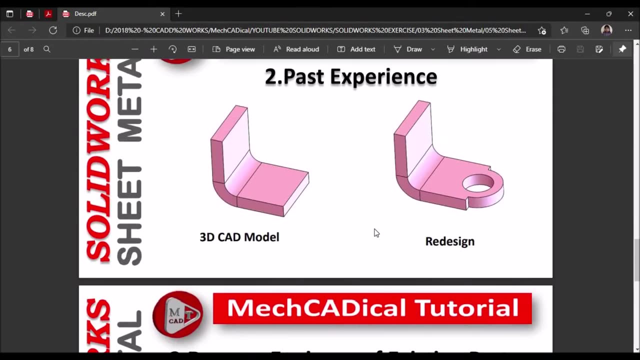 as per our requirement. So if we have previous experience on any component, it's easy to modify In the next step. we will create a new component And this is the design, So we can do earlier. design of the component. This is the design of the component, So we can do earlier design. 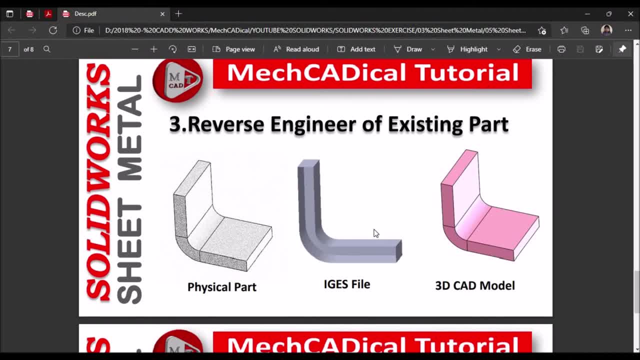 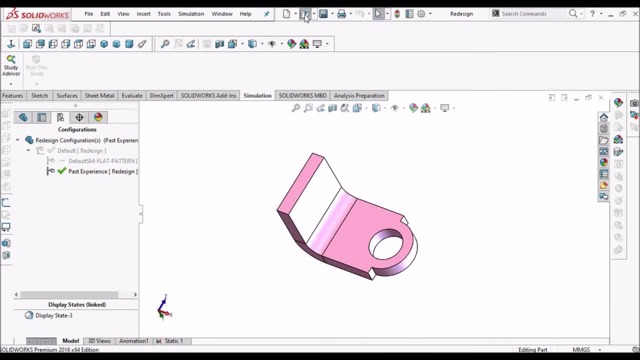 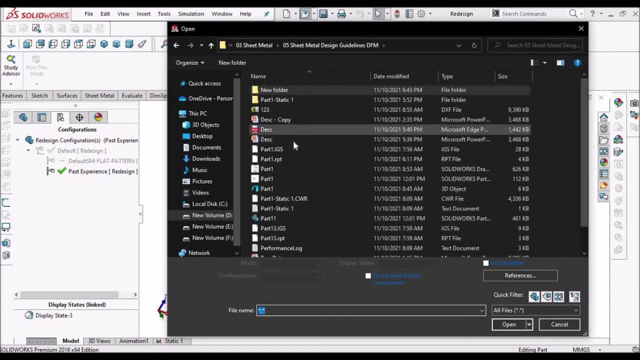 of the component. So we can do earlier design of the component and the next step is reverse engineering. So for reverse engineering, we will scan the component by laser scanning or white lane scanning and convert that file into an IGS file And we will import this file into the.